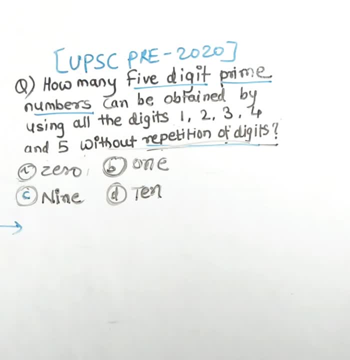 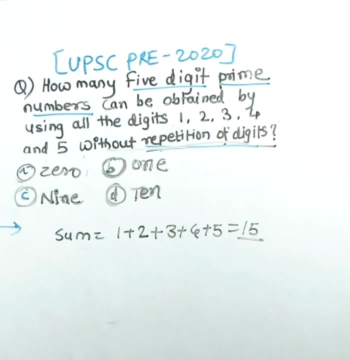 In this question we have to form 5 digit prime number using given digits and repetition of digits are not allowed. That means no digit can use twice in a single number. So now check sum of that 5 digits. That is 1 equal to 1 plus 2 plus 3 plus 4 plus 5 is equal to 15.. If you exchange their places, the addition will be the remain same, That is 15.. 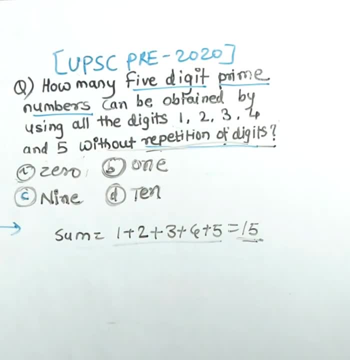 That is 15.. That means every number formed by these 5 digits always has. sum of their digits is equal to 15 and 15 is divisible by 3. That means every number formed by these 5 digits will be divisible by 3.. 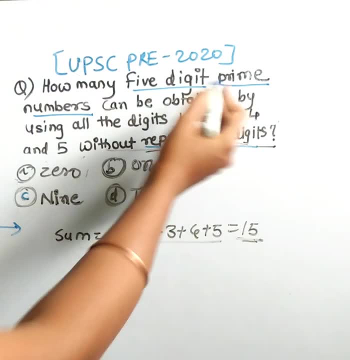 Therefore no 5 digit prime number will form, So our answer is equal to 15.. 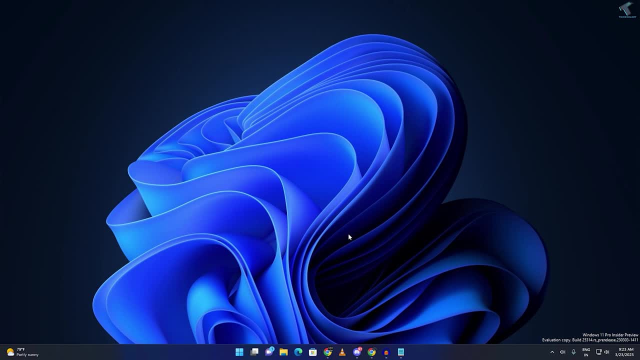 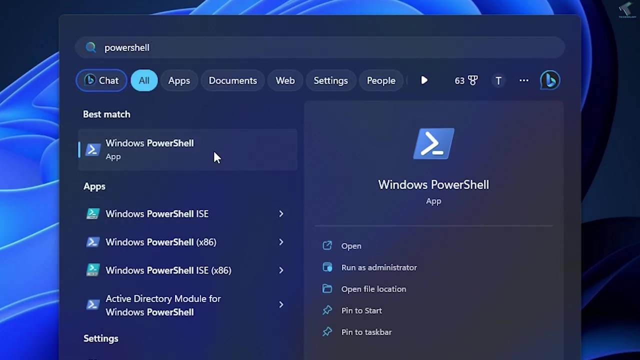 Hey guys, welcome back to my channel technology, and today, in this video tutorial, I will show you guys how to run a computer performance benchmark test on your Windows 11 PC or laptop. So you just need to follow me. So in this method, you don't need any third party software. You can use your PowerShell to run this test. For that you just need to go to your start menu, Type over here PowerShell. Now right click on PowerShell, Windows PowerShell and click on run as administrator. Click on yes After. 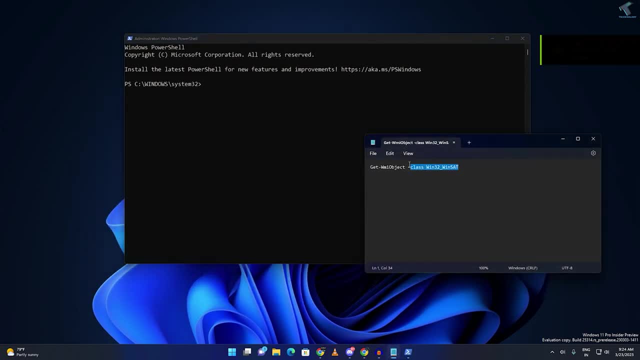 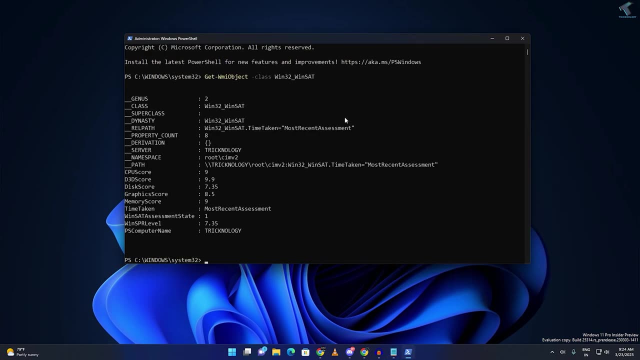 open PowerShell. you just need to copy paste this command from my video description, So I will give you the command on my video description. After that right click. after copy, Now press enter and here you will get a different types of score. as you can see, CPU score is 9.. In my case, graphics score and memory score. So I hope this quick tutorial will really help for you and please don't forget to click on the subscribe button, like button and share button, And if you have any questions or questions, then comments down below. I will see you guys.